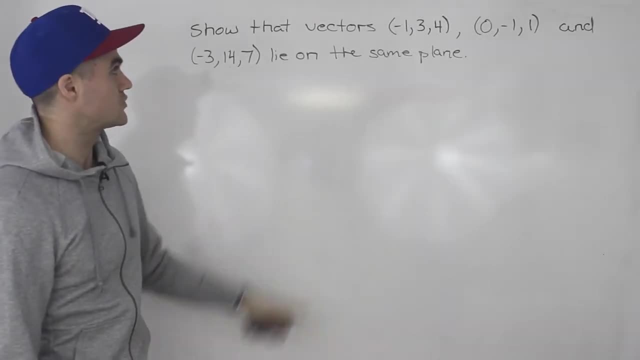 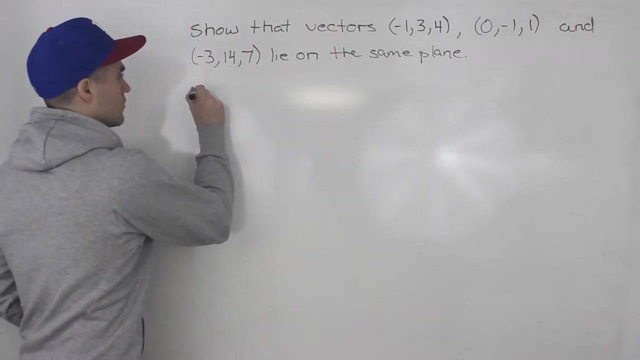 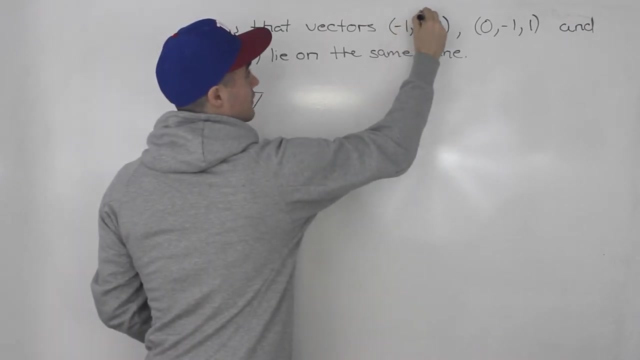 Welcome back everybody, Patrick, here. Moving on to the next question, we have to show that these three vectors here lie on the same plane or they are coplanar. So the way it looks visually, we got to show that these three vectors. let's say, this is vector A, this is vector B. 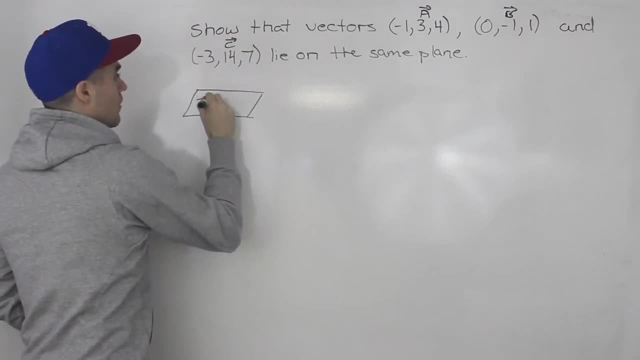 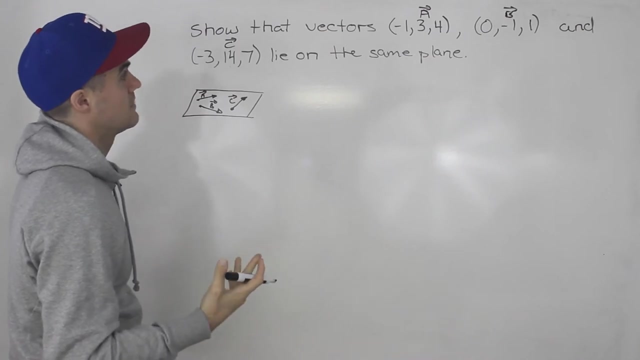 and then this one is vector C. We got to show that all three vectors are going to be coplanar or they lie on the same plane, And we went over how to do this in lecture videos. The way you do that is, you want to show that one of the vectors can be written as a linear combination of the others. 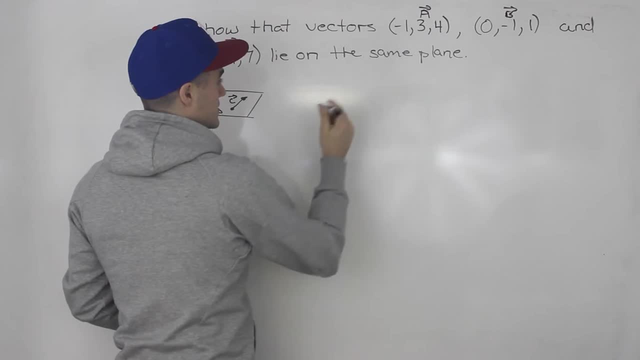 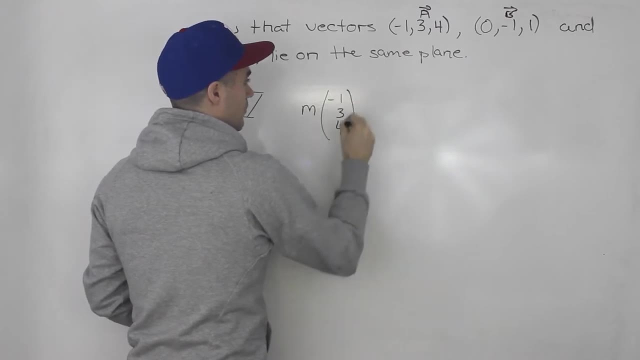 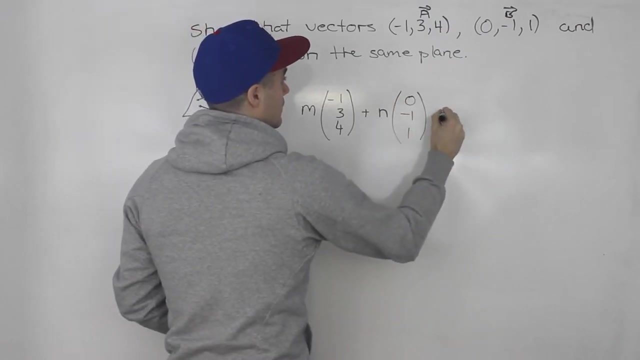 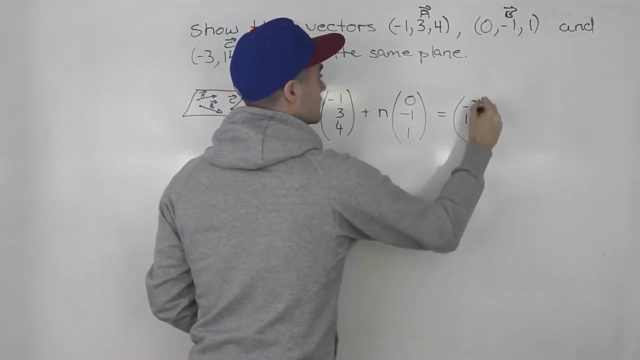 So let's show that if we take a constant m, multiply it by vector A, plus a constant n multiplied by vector B, so 0, negative 1, and 1,, we can get this vector here negative 3,, 14, and 7.. Now we could have also switched this up. 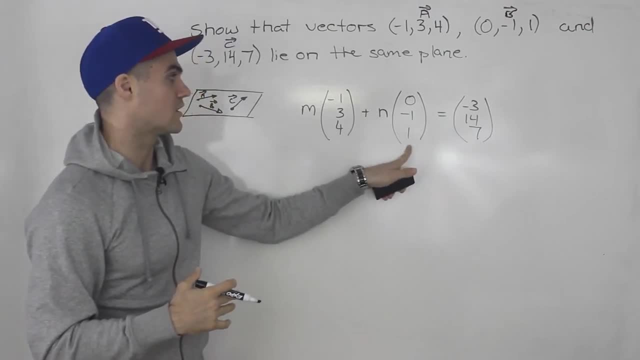 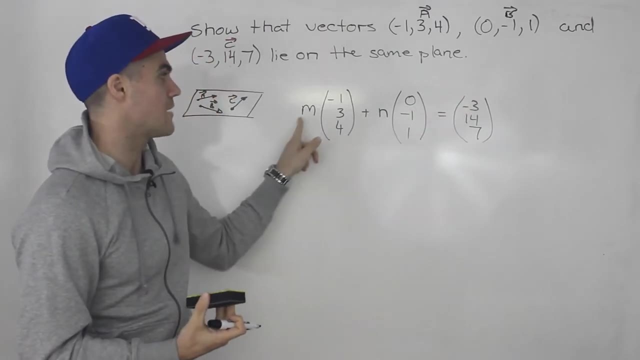 so we could have maybe even put this vector here, this vector over here. Personally, I like to take the vector with the biggest numbers and put it here, because then when you solve for that m and n, there's a smaller chance that you're going to be working with fractions. It's not guaranteed. 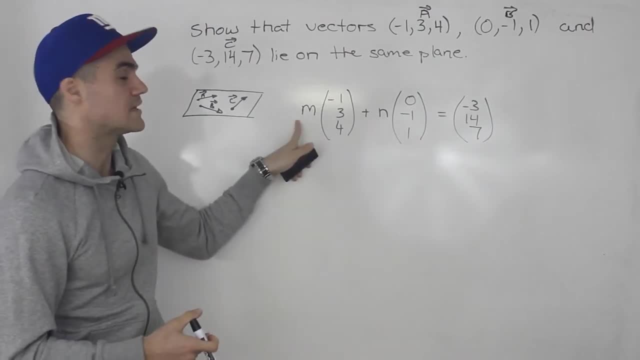 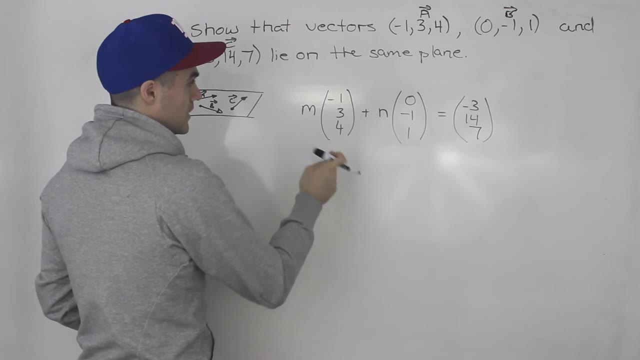 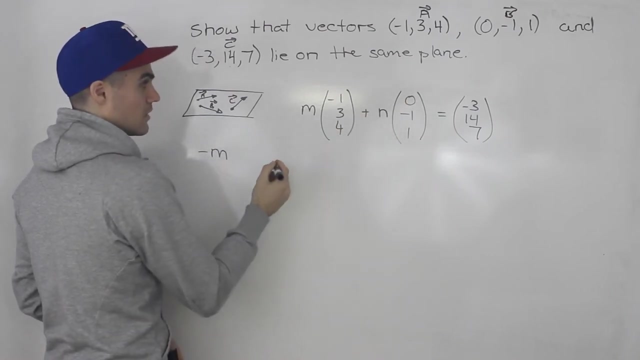 but it's a higher probability that these will be integers that you're working with. So now we have this set up, we can make three equations. So m times negative 1, that is negative. m n times 0 is just 0, and then this has to equal negative 3.. m times 3,, that is 3m. 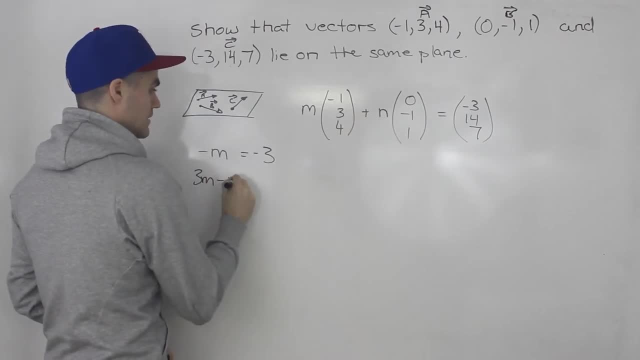 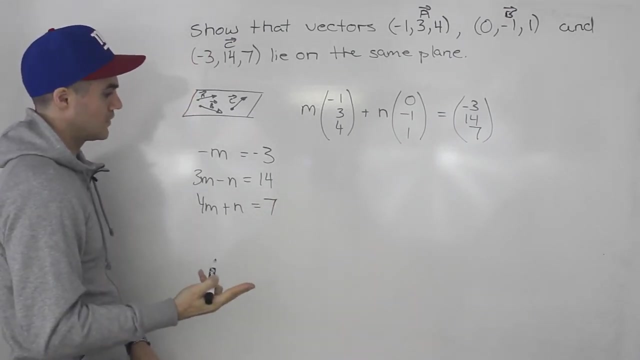 n times negative. 1 is minus n, that is equal 14, and then 4m plus n has to equal 7.. Right, So we got three equations, but we only have two unknowns, So we only have to pick two of the.